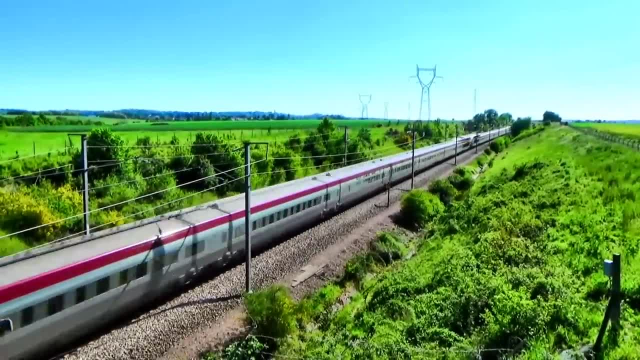 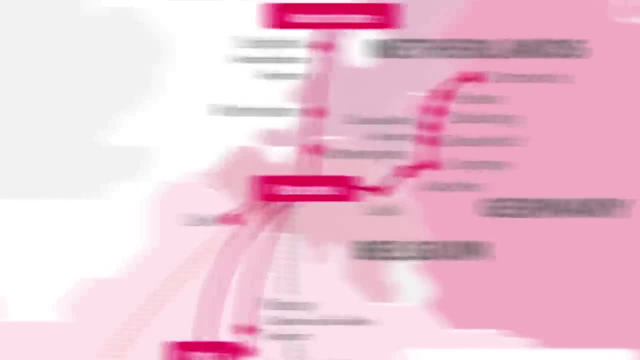 one of Europe's finest ever since its first launch in 1997.. The Thales makes its stop in great capitals such as Paris, Brussels, Amsterdam and London. The train rides at a speed of 186 miles per hour, or 300 kilometers per hour, and is Europe's. 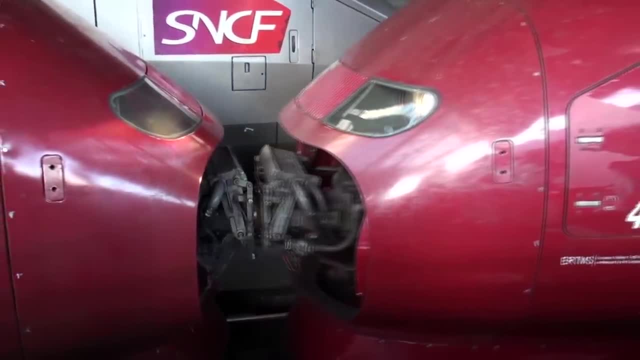 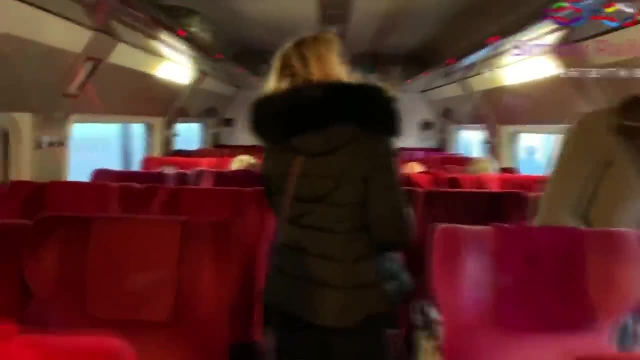 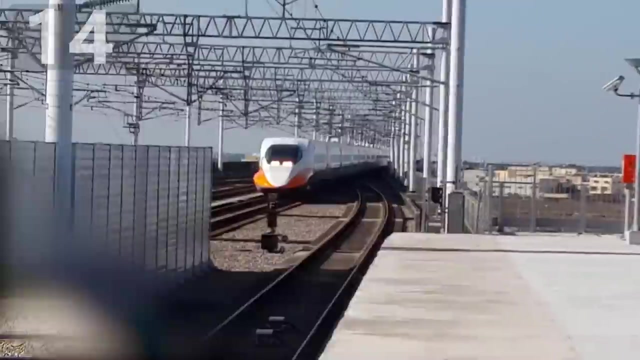 first sustainable and pro-green train. With over 7 million passengers annually, the Thales remains to be one of the most popular modes of transportation And, while this train has several destinations all around Europe, its signature train line is from Paris to Brussels, Number 14,, THSR-730.. 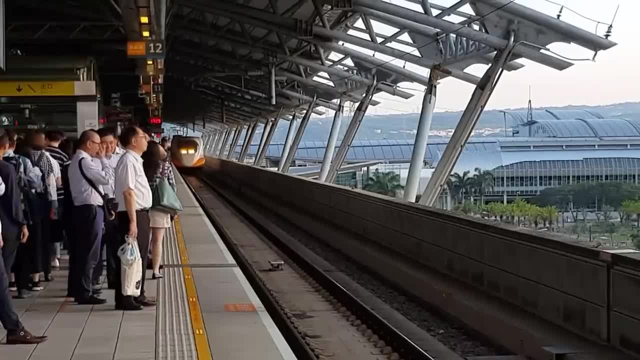 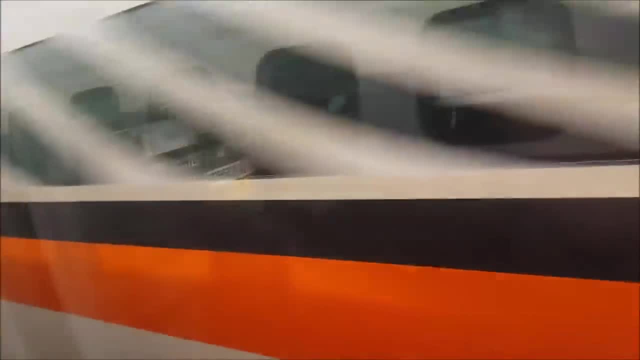 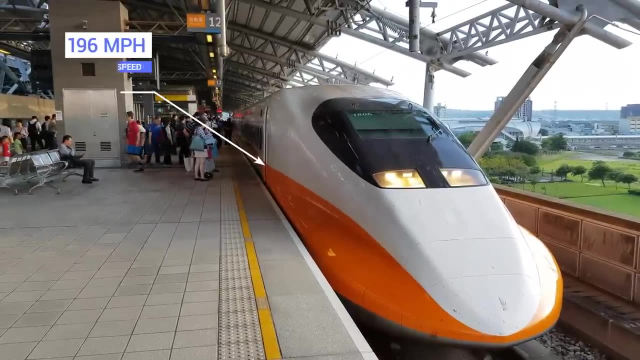 700T, 196 miles per hour, Taiwan's fastest high-speed train, was introduced to the world in 2007.. The THSR-700T is a blend of world-renowned Japanese train manufacturing companies, and its speed can reach a maximum of 196 miles per hour, or 315 kilometers per hour With 12 carts. 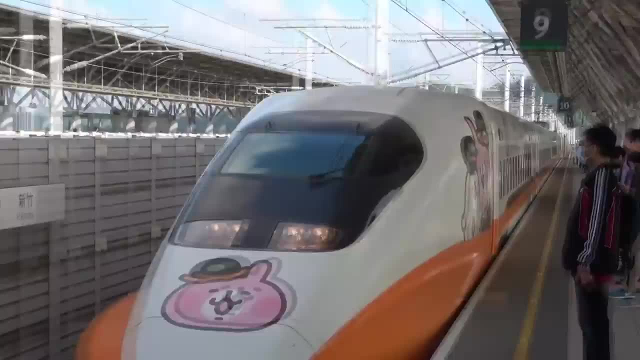 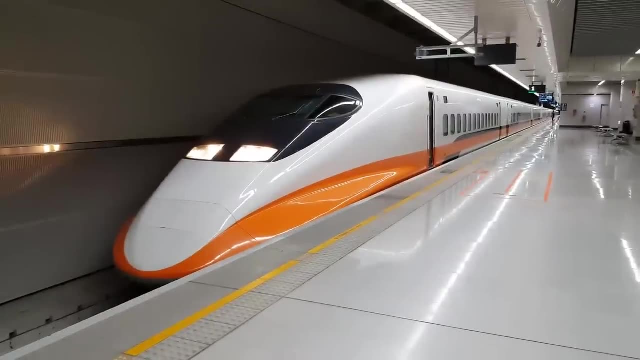 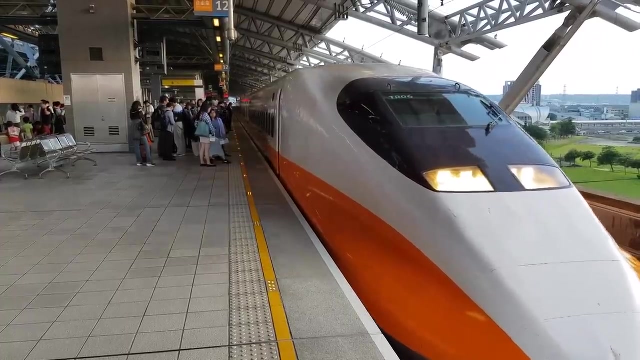 seating capacity of transporting 989 passengers at a time, the 700T is Taiwan's go-to transit choice. Unlike other Japanese constructed high-speed trains, the THSR does not feature an aggressive aerodynamic nose design and instead is focused to optimize and maximize seating capacity. 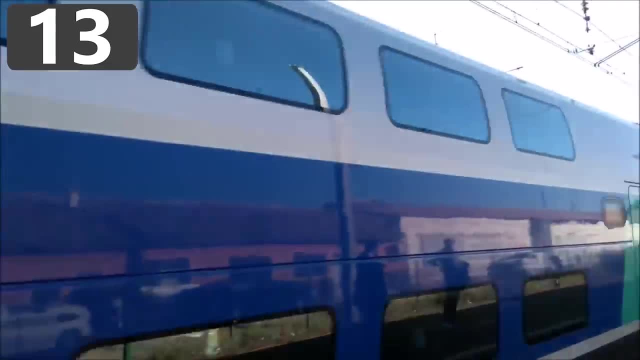 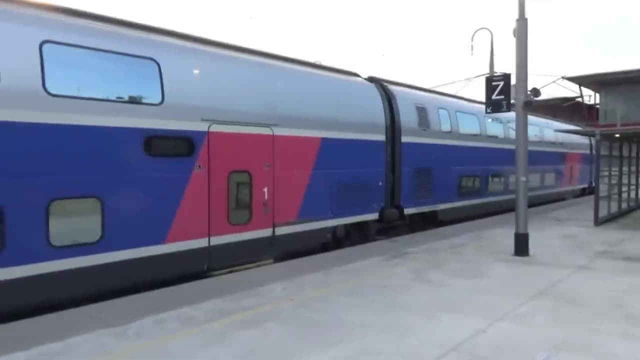 Number 13,: Alstom EuroDuplex- 198.8 miles per hour. The Alstom Avelia EuroDuplex, known simply as EuroDuplex, is another example of Europe's finest high-speed trains. The train is operated by the French railway company SNCF. 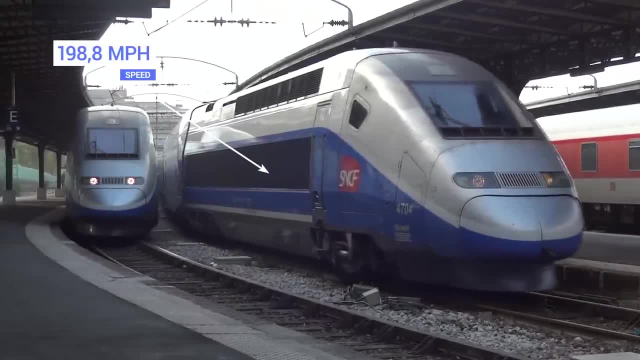 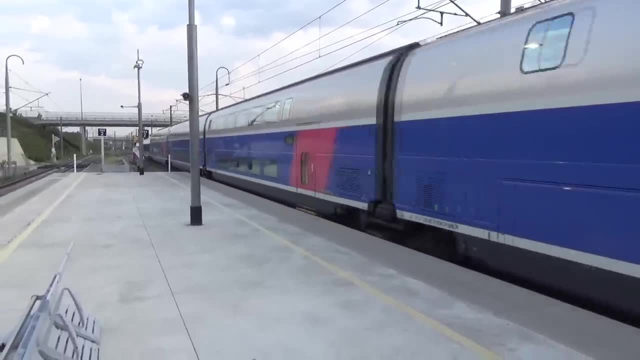 and has a maximum speed of 198.8 miles per hour, or 320 kilometers per hour. The train, that can transport 1,065 passengers at a time, is known for its light body weight and impeccable aerodynamics, Traveling through France, Luxembourg and Germany. 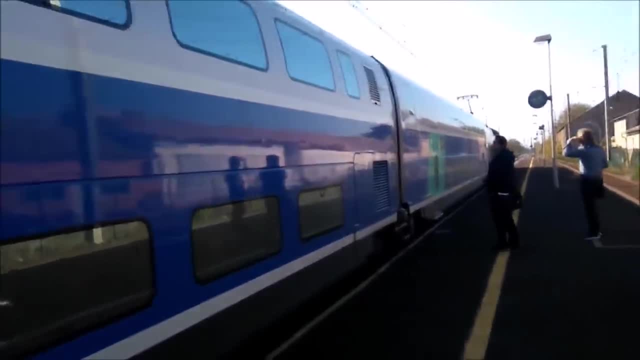 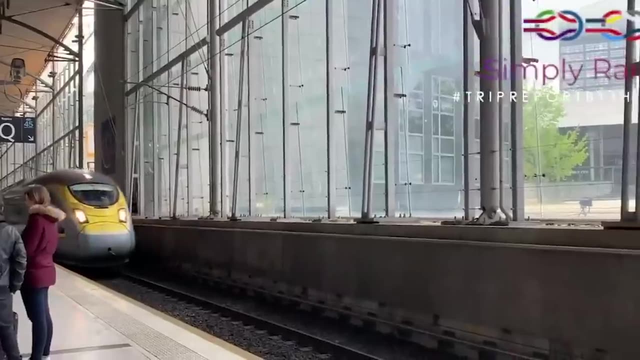 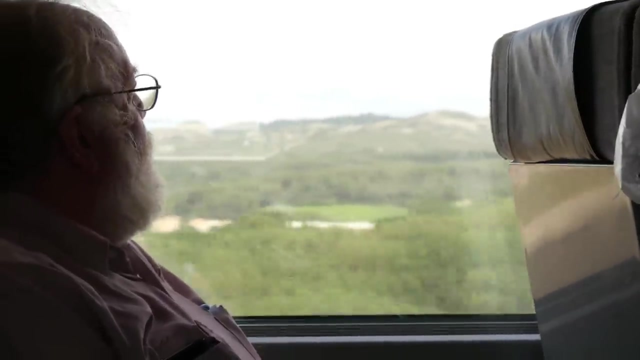 the EuroDuplex is a great choice for intra-country transport. Number 12,: Eurostar E320, 200 miles per hour. Just like the EuroDuplex, this British high-speed train is another popular choice amongst travelers. The Eurostar E320 first began its service in November 2015,. and can swift at 200 miles per hour or 321 kilometers per hour. Running through the Eurotunnel, this high-speed train has connection lines in London, Paris and Brussels. With a capacity of 900 passengers, it's equipped with a regenerative braking system. 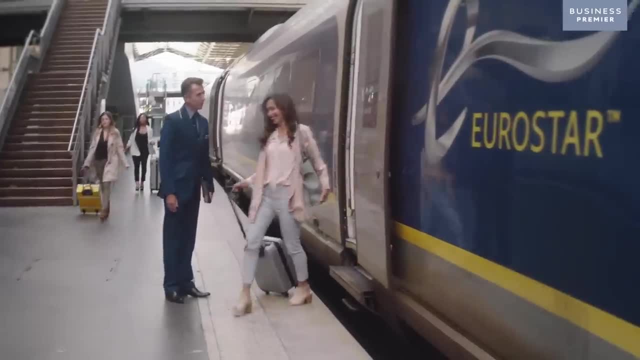 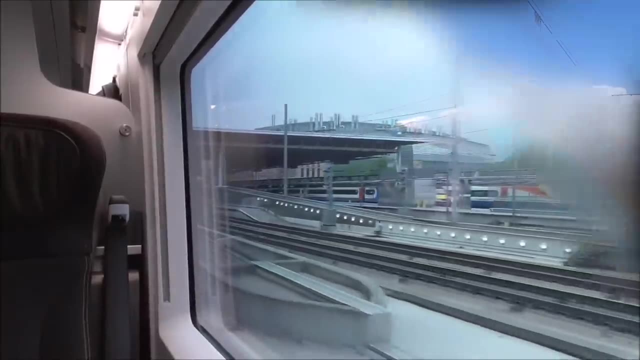 The Eurostar E320 is 400 meters in length and with ticket prices less than 100 bucks, it's no surprise that many prefer traveling with high speed and affordable trains. Number 11, CoreRail KTX, 205 miles per hour. 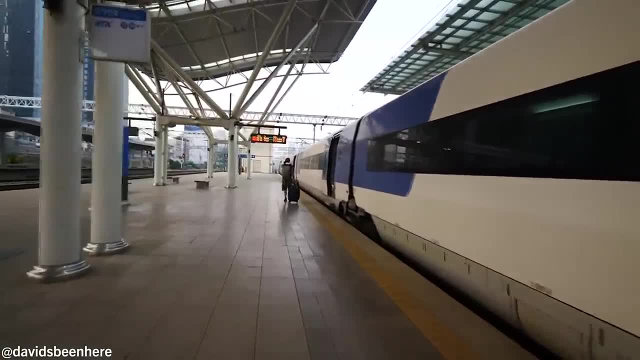 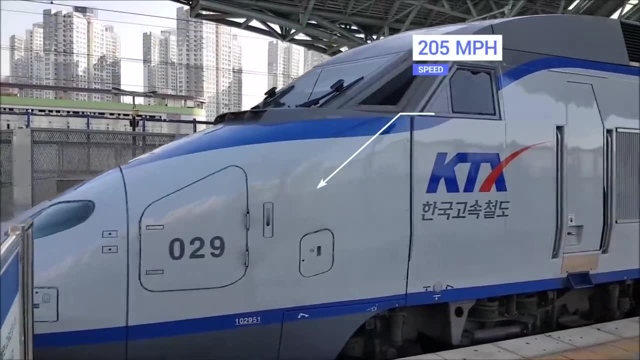 The CoreRail Korea Train Express, or KTX, is South Korea's fastest train up to date, With nearly 12 years of construction. the KTX runs at the speed of 205 miles per hour, or 330 kilometers per hour, and has been in service from 2004.. 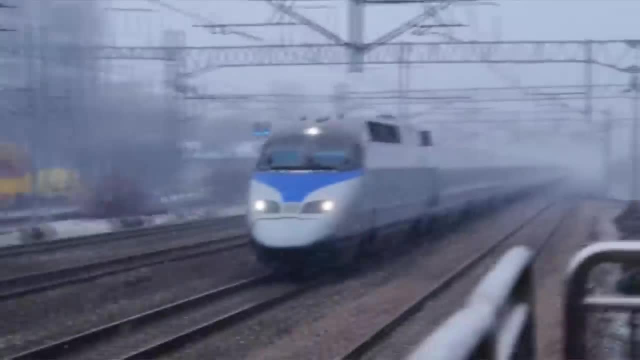 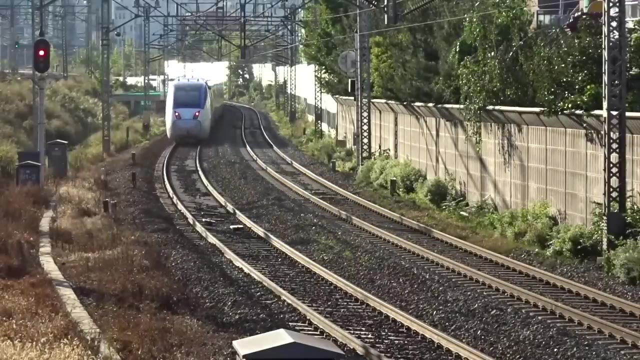 Capable of carrying up to 935 passengers, this fast train is ergonomically built, suited to fit the body shapes of Koreans. with individual passengers, Individual cinema sets on every seat, vending machines at arm's length and comfortable seating, The KTX proves to be a preferred choice over air travel. Number 10,: Deutsche Bahn ICE, 205 miles per hour, Traveling at the same speed as the CoreRail KTX. the Deutsche Bahn Intercity Express, or just ICE, is Germany's finest, Operated since 1985, the ICE can travel at 205 miles per hour. 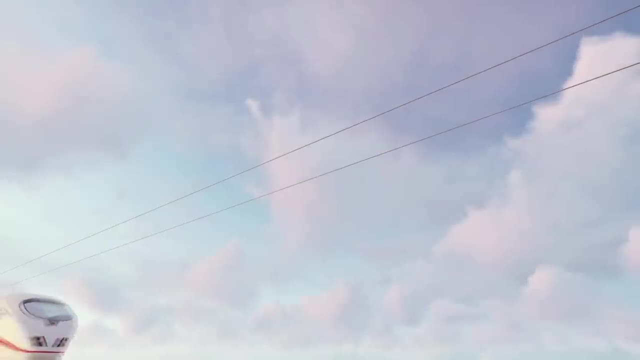 or 330 kilometers per hour. And we have to mention that it is a 4- Zarrow station which is located on the outskirts, All of those regions around Die Heide, all of which are occupied by Germany and are also part of Berlin. 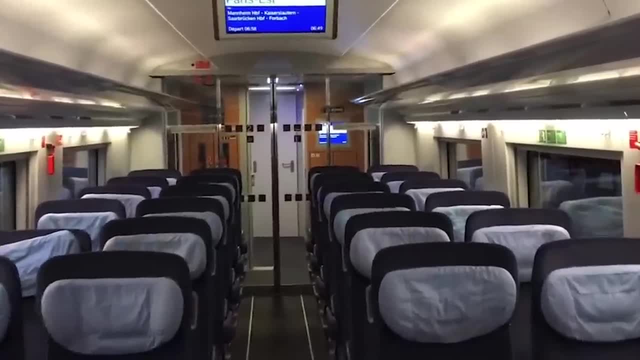 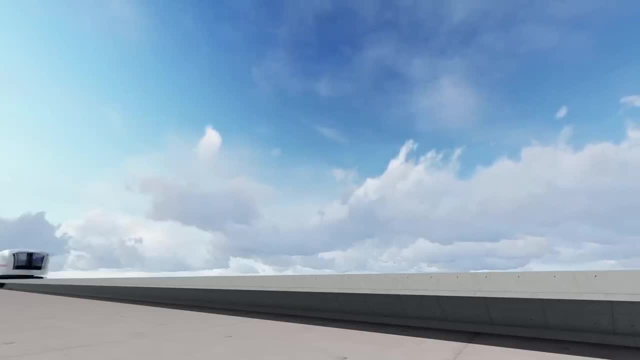 The ICE has traveled through Germany, but is not the only one with connecting lines. in Denmark, this swift train carries around 2 billion passengers every year. With its futuristic exterior design, the ICE was awarded the Red Dot Design in 2015,. 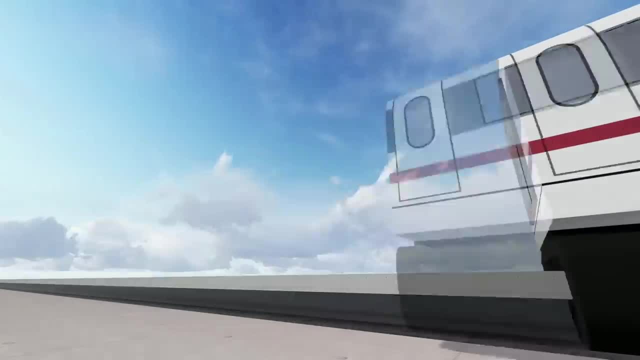 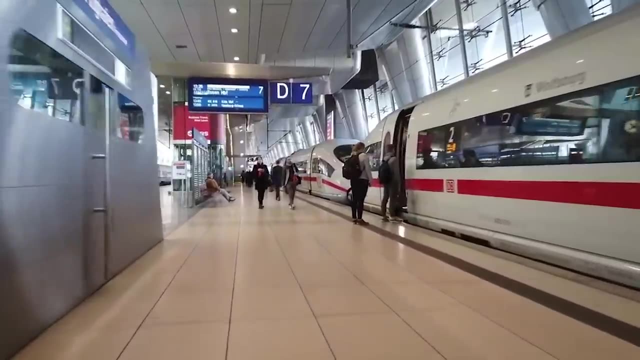 and is the go-to choice for visitors and passengers all over Germany, Even on long stretches such as Berlin to Basel, which takes around eight hours of journey time by train, especially if it's of a high-speed caliber, With mostly inter-country travel and. 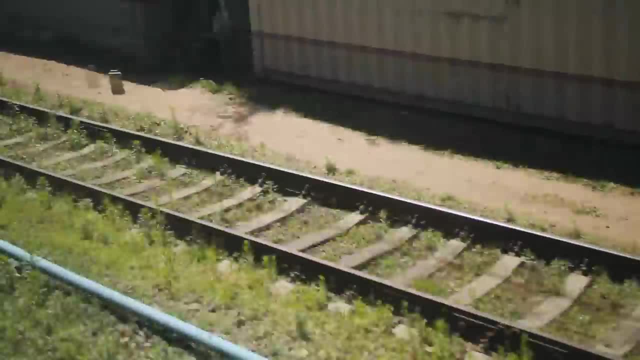 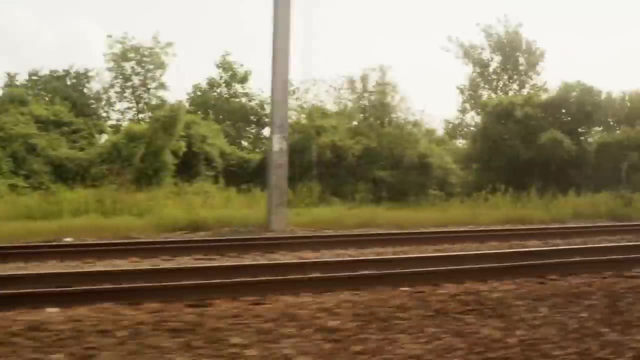 some routes expanding into neighboring countries. the Deutsche Bahn and ICE network has a capacity to send off 280 trains per day. These frequent voyages are another reason why travelers from all over the world prefer comfortable train rides over anxiety-inducing air travel. 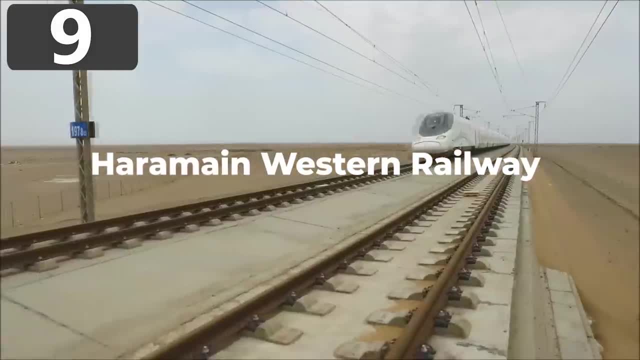 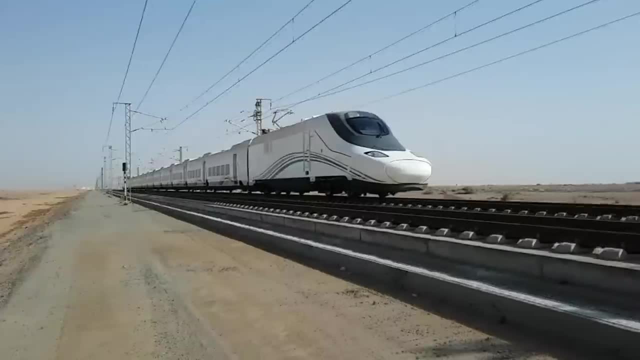 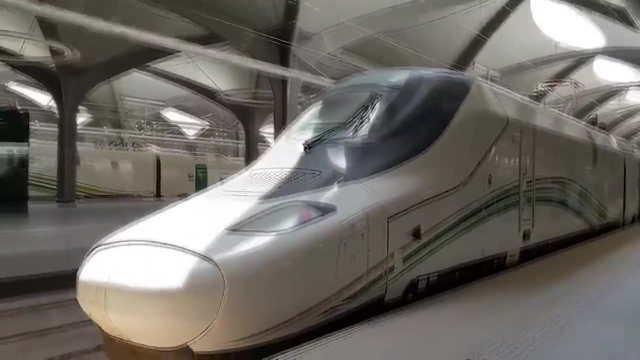 Number 9. Haramain Western Railway. Known as the Western or Mecca-Medina Railway, the Haramain high-speed train is Saudi Arabia's best. With nearly a decade of construction and assembly, this train costs a shocking $9.4 billion to build. With a speed of 217 miles per hour, or 350 kilometers per hour, the Haramain Western is the 10th fastest high-speed train in the world. The train can transport 417 seated passengers at a time, and it's estimated to carry around 60 million travelers every year With its 217 passengers per hour. the Haramain Western is the 10th fastest high-speed train in the world, With its 217 passengers per hour. the Haramain Western is the 10th fastest high-speed train in the world, With its 217 passengers per hour. the Haramain Western is the 10th fastest high-speed train in the world. With a speed of 180 miles or 450 kilometers, the Haramain were closer to a walled AmTA platform. This $9.4 billion dollar train needed 9 years of non-stop construction, and its arrangement was divided into two phases, Phase one consisting of designing, planning and starting. 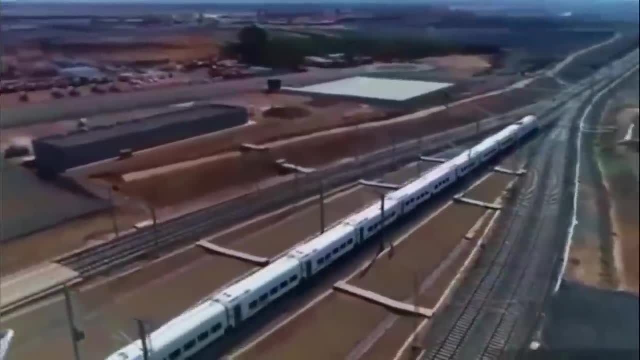 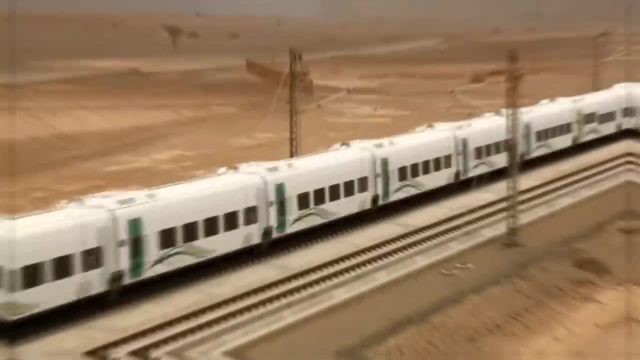 construction of the finished product. By the end of Phase one, around $2 billion dollars was spent in assembling four of the 5 stations to build the Haramain Western. Phase two dealt with the remaining infrastructure obstacles such as train power, partie space and readily available free. 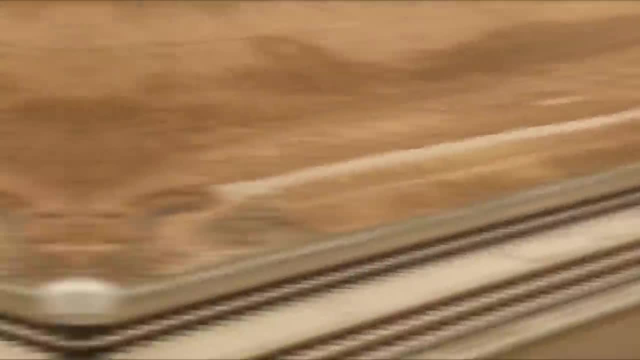 power. Phase two dealt with the remaining infrastructure obstacles, such as train power, electricity and signaling. Anticipated to have started its services in 2012,, the construction and design took longer than expected and the final Jaramain Western train was opened to the 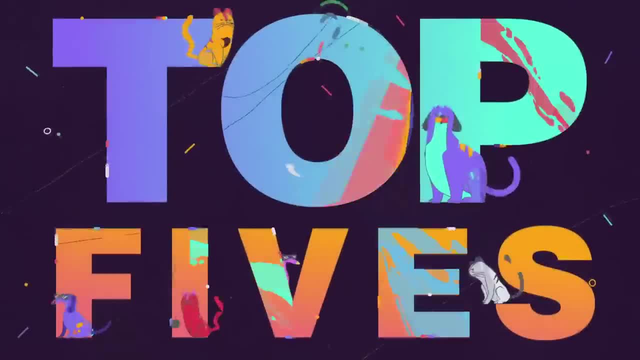 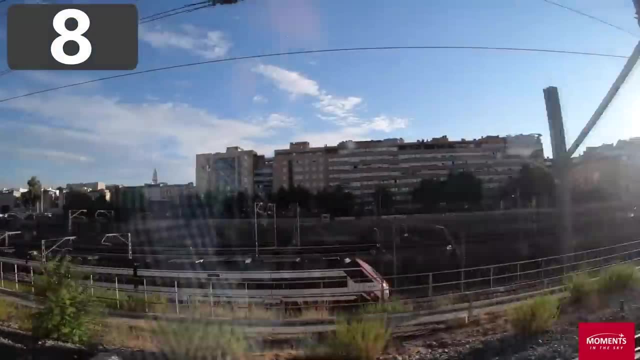 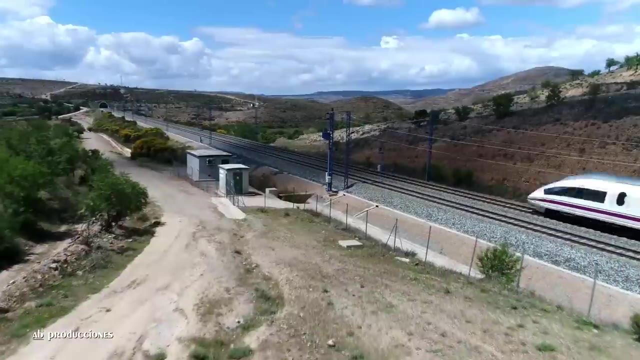 public in 2018.. Before we move on, be sure to subscribe to Top5s with notifications on Number 8.. Renfe AVE. Some of the fastest trains in the world belong to the Spanish Renfe Alta Velocidad Española, or just AVE, train service, The high-speed trains. 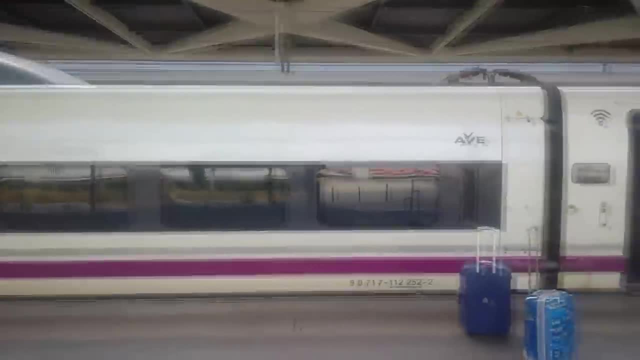 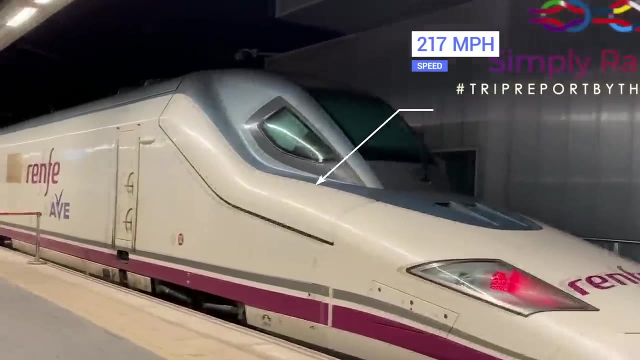 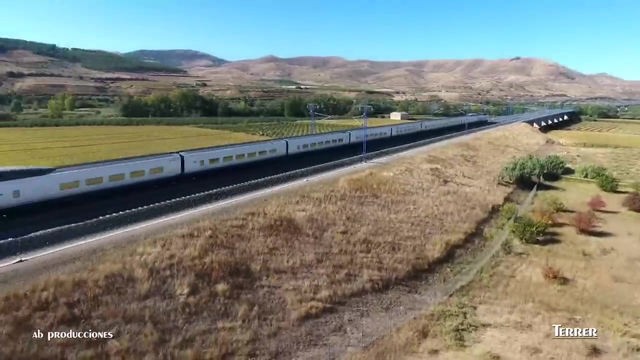 that have been operating with the ACE service ever since 1992 have the same speed as the Jaramain Western. With a 217 mph or 350 kmph speed under its belt, the Renfe transports around 20 million passengers every year, A train that literally translates to Spanish High Speed, or BIRD. if 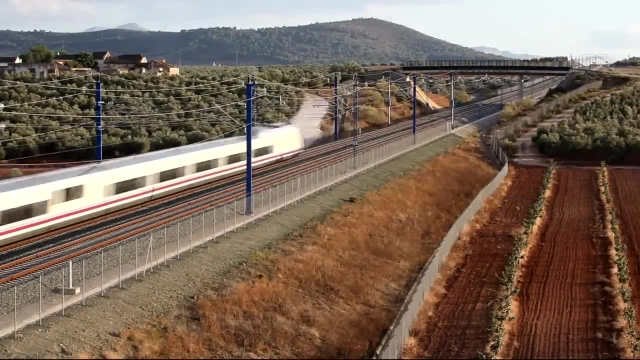 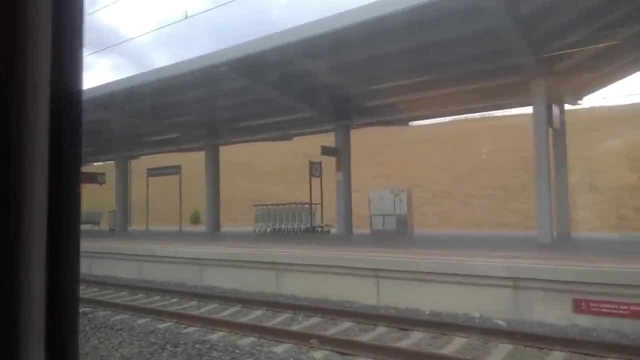 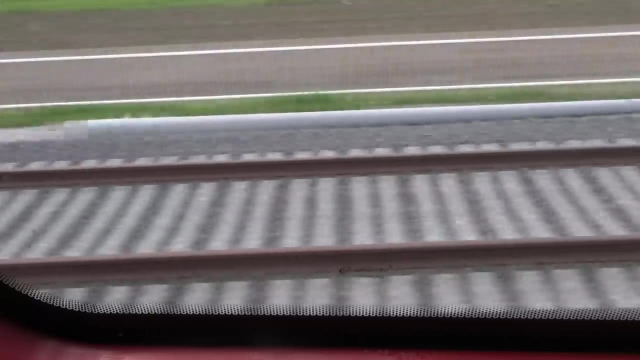 links all over Spain and even some lines in France As of 2020,. the Spanish AVE system is the longest high-speed railway network in Europe: Its 2,010-mile or 3,200-kilometer railway line is also the second-longest in the world, coming in shorter than China. 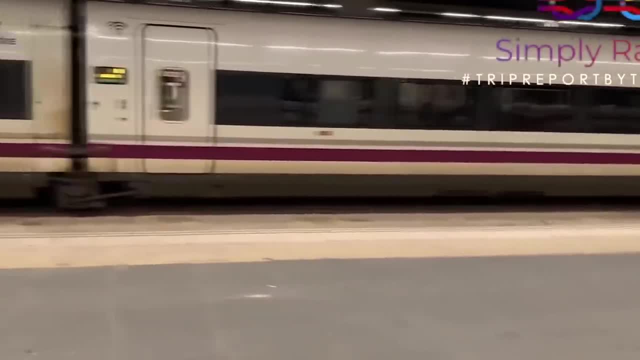 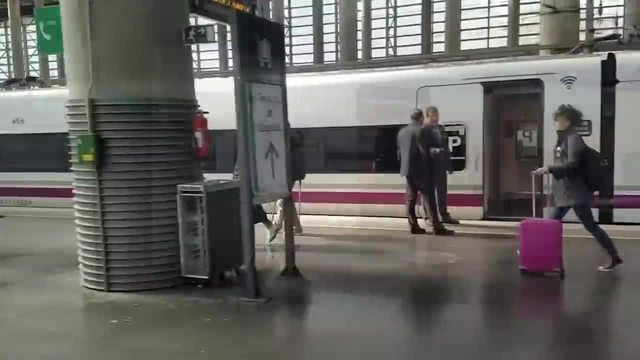 When it comes to specific trains, the Renfe company bought several first-class operating trains for their successful transport lines. Built by the German industrial conglomerate Siemens Velaro, it's a family of high-speed trains that travel all across Europe, with connecting points and lines in Germany, Belgium, France, the UK, China. 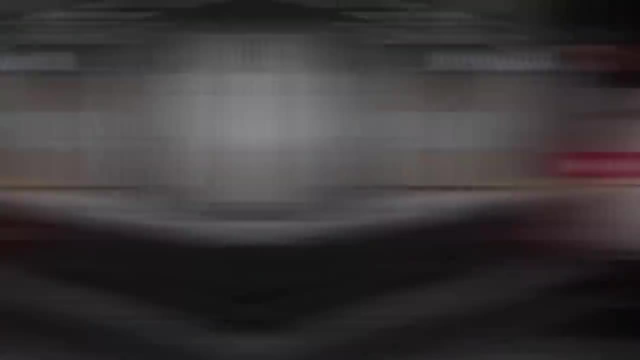 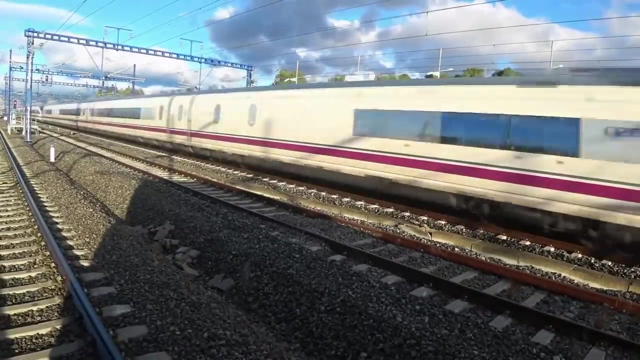 Russia and Turkey. The Siemens trains have some of the vast variety of intercountry transport. When it comes to the fastest of the family, the Velaro E103 is the swiftest of them all, With cheap and inexpensive ticket prices starting at 32 euros or 65 bucks. traveling and exploring. 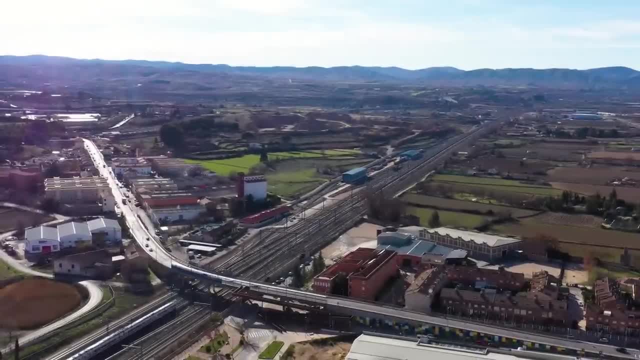 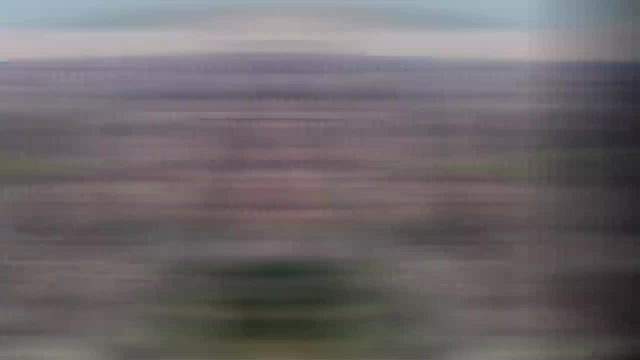 Spain can be fun and affordable at the same time In the upcoming years. there are more than 10 new train lines that are currently under construction and will soon start to operate, Expanding all throughout the beautiful country of Spain. visitors and tourists traveling. 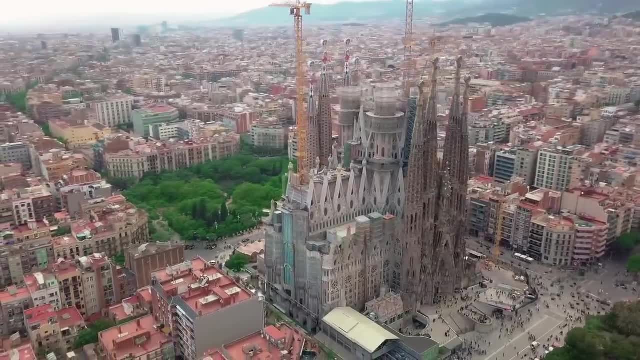 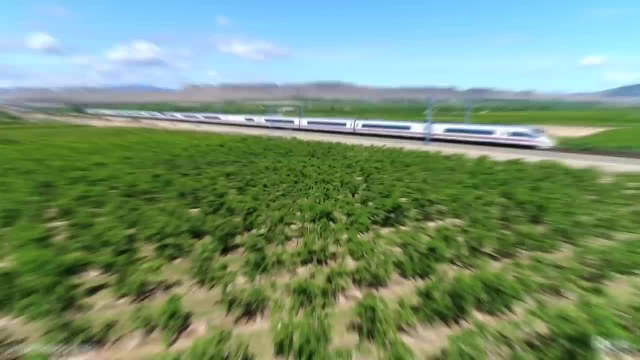 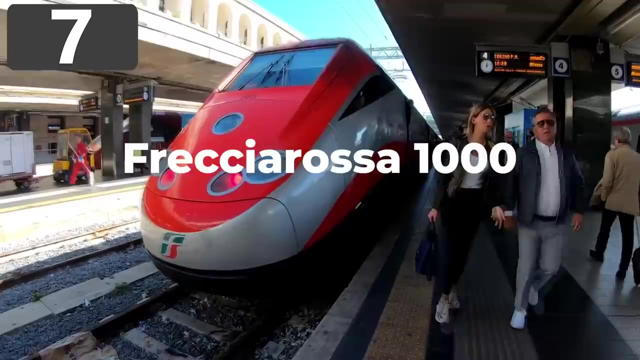 with the AVE will be able to get on board. If you ever decide to take a road trip across Spain, remember to keep Renfe AVE as your mode of transportation at the back of your mind. 7. Frecciarossa 1000. 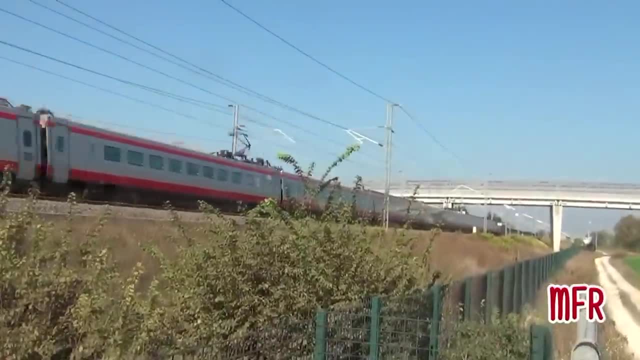 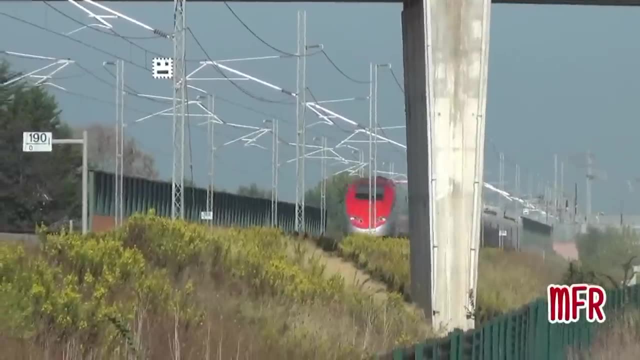 Europe's fastest high-speed train is the Frecciarossa 1000, also known as the ETR 400.. This high-speed train is operated by an Italian railway company and has a maximum speed of 220 miles per hour. The ETR 400 is the fastest high-speed train in the world. The ETR 400 is 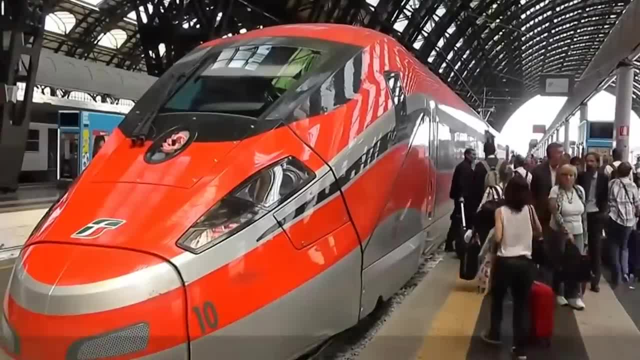 the fastest high-speed train in the world. The ETR 400 is the fastest high-speed train in the world. The ETR 400 STARTS AT 144 Kms, or 354 kilometers per hour. Europe's finest and greatest train started its construction in 2008.. After years of 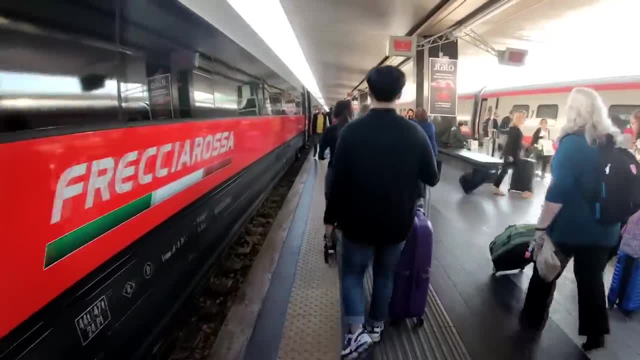 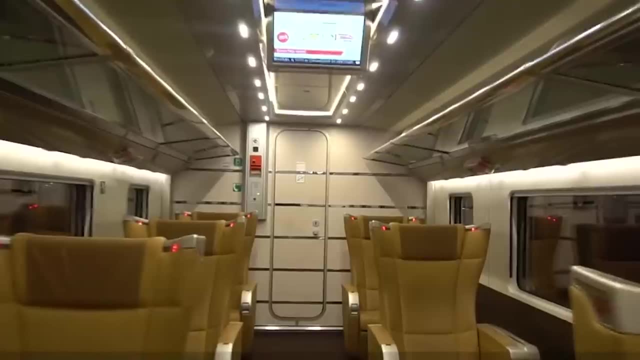 careful assembly and the impeccable building Frecciarossa was finally open to travelers in 2015.. Operated by Trenitalia, the ETR 400 offers maximum comfort to visitors and tourists who want to explore Italy in its prime. The 660-foot or 202-meter-long train is made of nearly 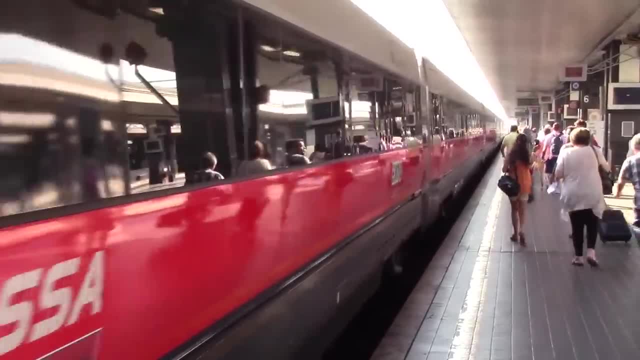 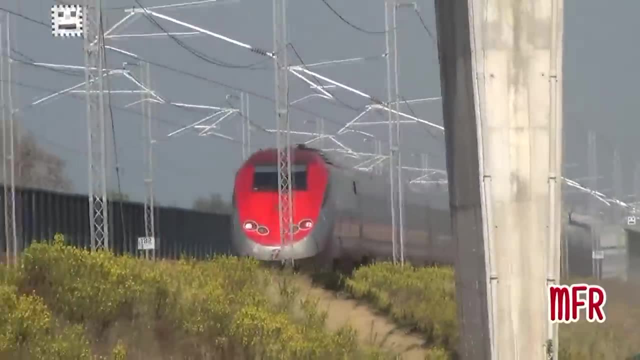 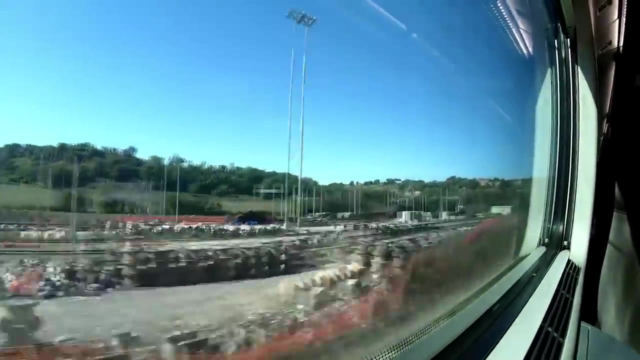 100% renewable and sustainable operating parts and components, making it one of the most friendly trains in the world. The Fracarossa has a characteristic long nose on its front end, which ultimately provides excellent aerodynamic properties, Designed specifically for optimizing shock absorption and maximum 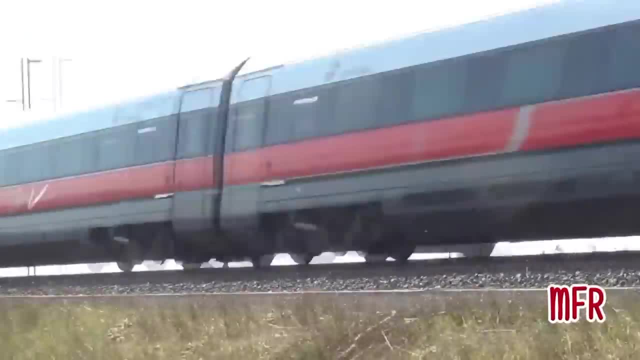 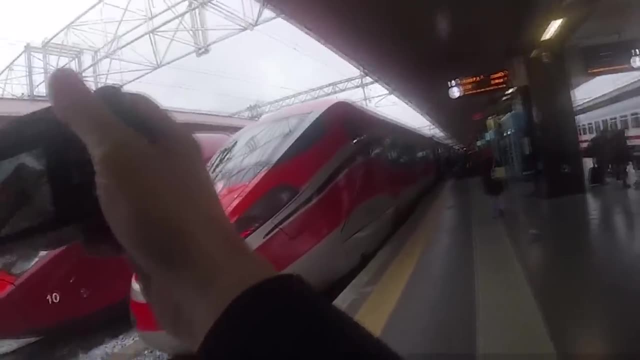 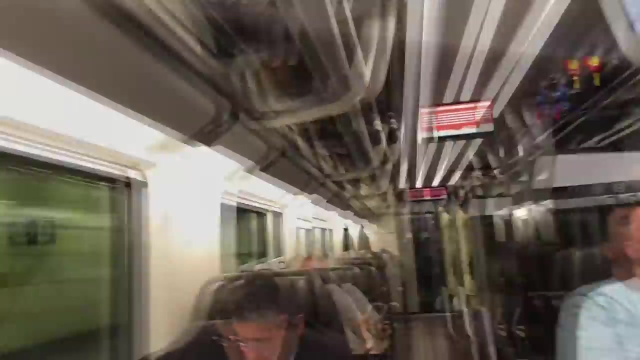 safety. this unique design aids in the train's overall function and, along with 16 powerful engines distributed all across the train's length, the ETR 400 can successfully reach its monumental speed. The Italian train's interior design is also remarkable for its special features, With wide corridors. 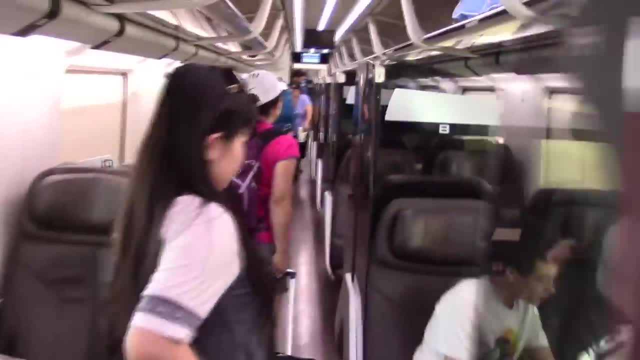 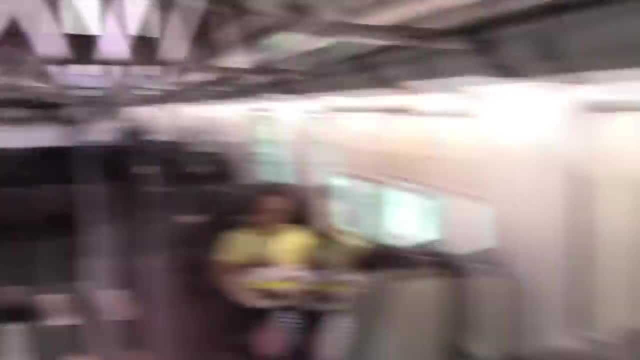 ergonomically shaped seats, 4G internet service and soundproof cabins. the ETR 400 is truly one for comfort and luxury And with 485 passenger seats available in four classes: executive, business, premium and standard- Europe's fastest. 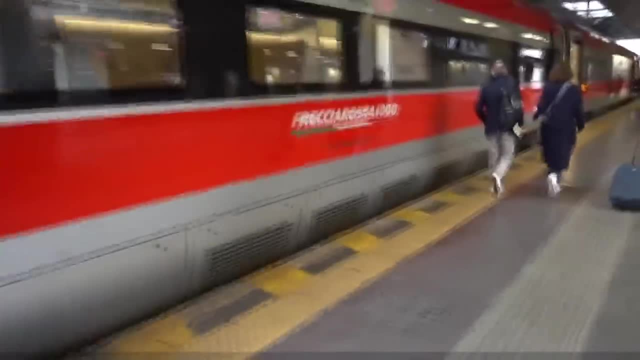 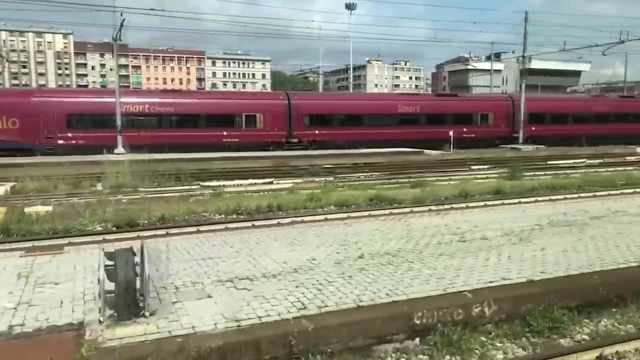 train offers impeccable ease and safety. Number six: AGV Italo: 223 miles per hour. AGV Italo is one of the fastest trains in the world, first in the world and the fastest in the world First undergoing prototype construction and assembly in the year 2000,. this train 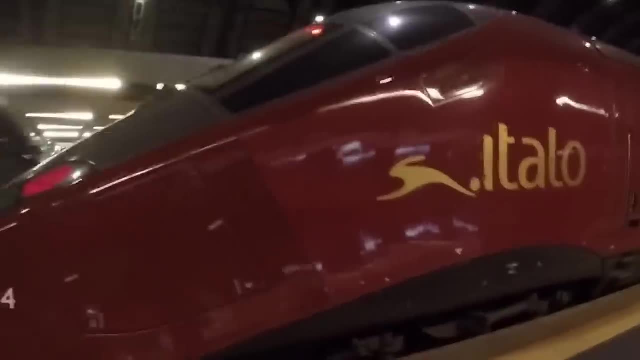 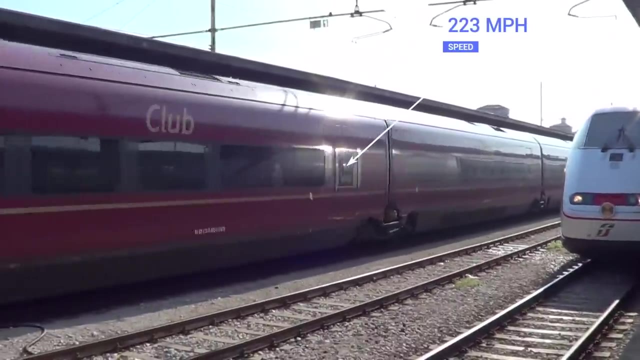 has come a long way from its initial release and operation. This fast train began its journey in 2012, and, as of 2020, the AGV has a maximum speed of 223 miles per hour, or 359 kilometers per hour, and is widely used amongst travelers in. 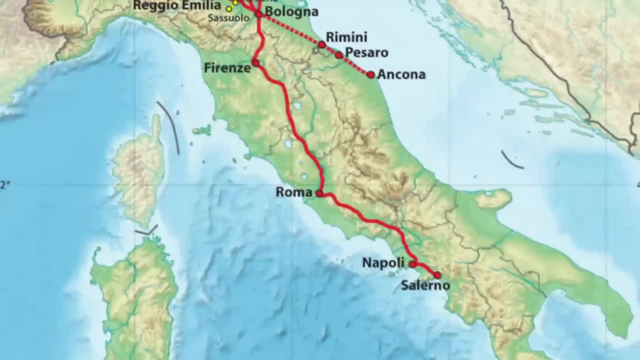 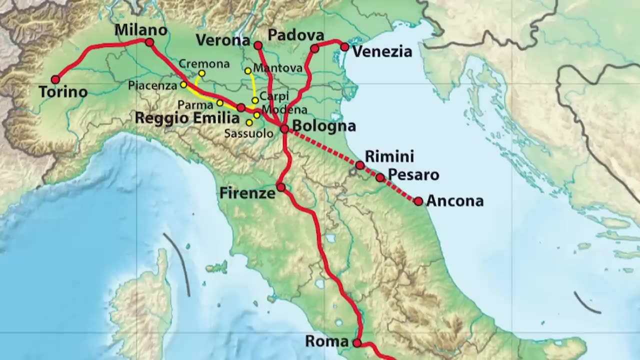 Europe. This mega speed train runs from Rome to Naples and covers about 140 miles, or 225 kilometers of distance, in less than one hour. Not only is the AGV one of the fastest trains in the world, but also one of the fastest trains in the world. 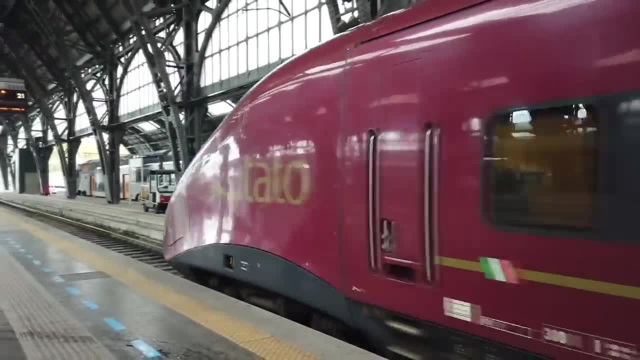 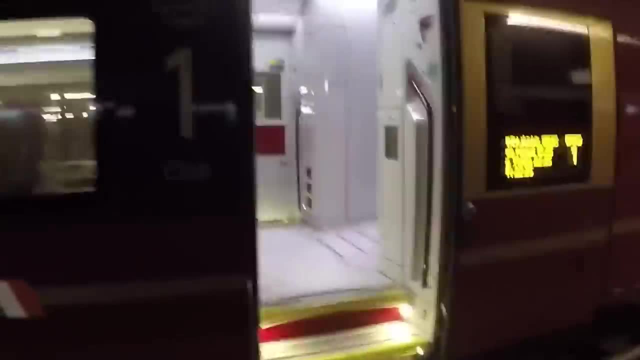 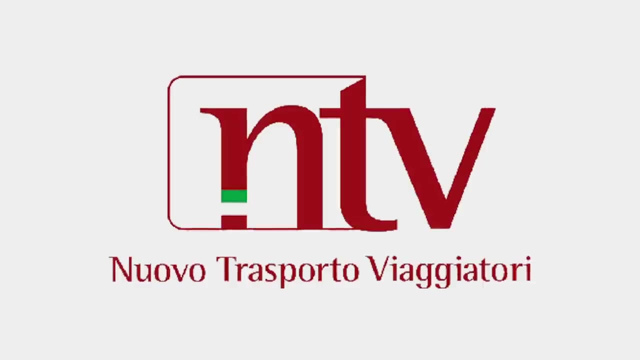 But it's also an eco-friendly construction work, as approximately 98% of its body parts are recyclable. Even though the AGV train was manufactured by the French company Alstom, it was purchased by the Italian company Nuovo Transporto Vigiatore, or NTV, in 2008.. Since then, 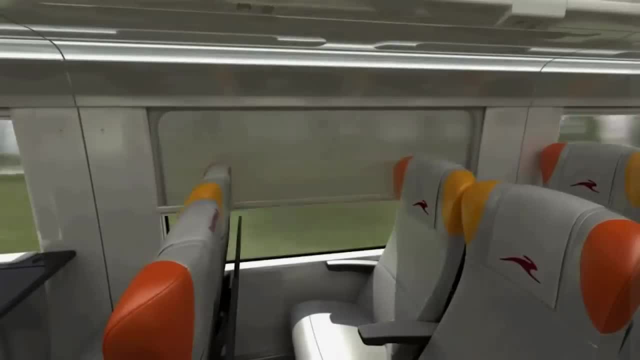 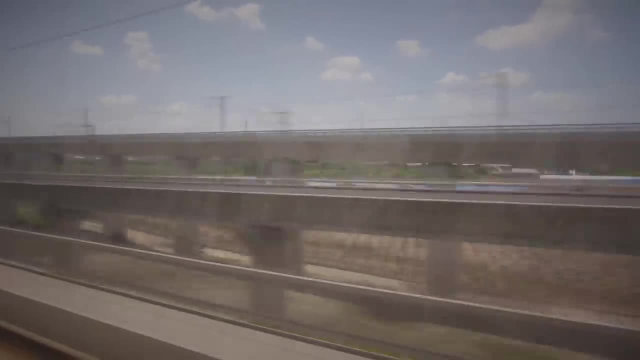 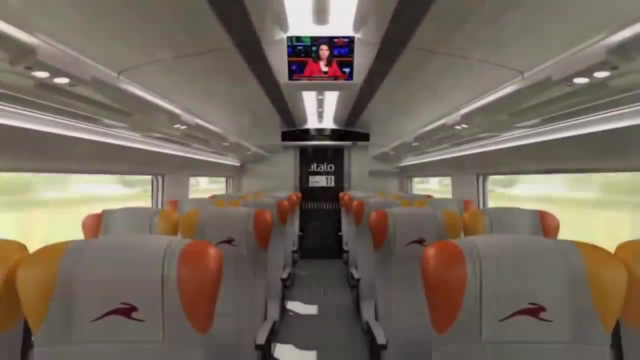 it's been regarded as the AGV Italo. It cost around 100 million euros to develop and construct, but the Italian conglomerate bought it for a hefty price tag of 650 million euros. The 430-foot, 132-meter-long train has seating to accommodate from 245 to 446 passengers at a time. 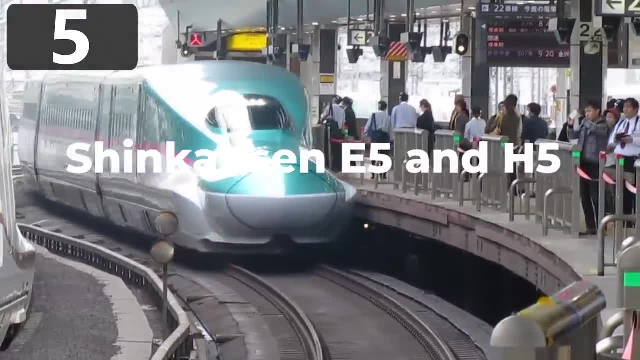 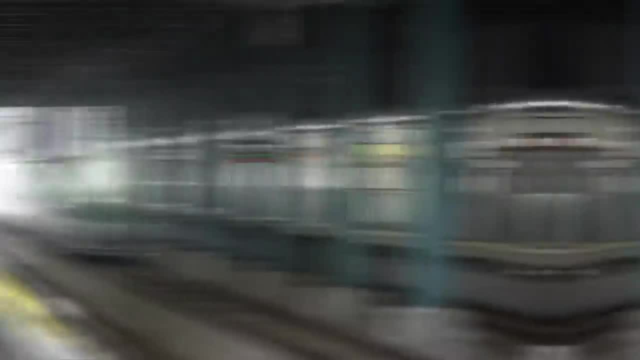 Number 5. Shinkansen E5 and H5, 224 miles per hour. When it comes to the fastest train in Japan, the award goes to the Shinkansen E5 and H5 series. These high-speed trains share the same maximum speed of 224 miles per hour. 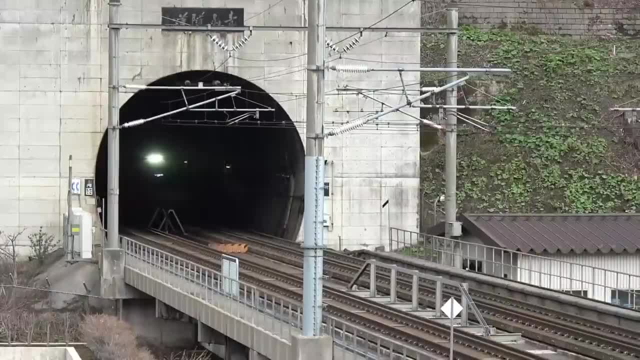 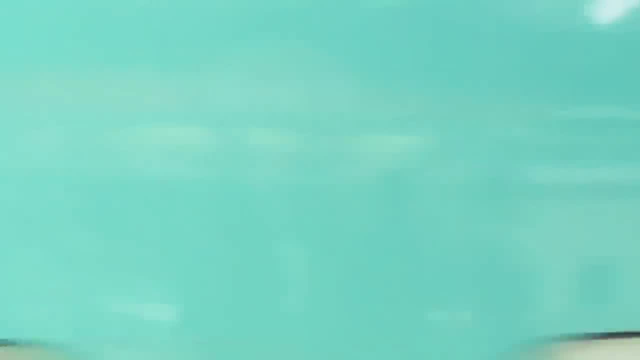 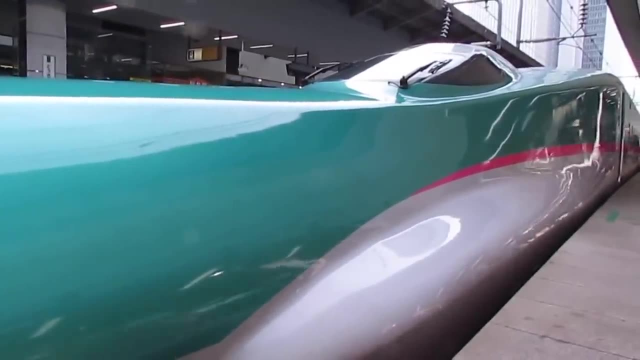 or 360 kilometers per hour, and were constructed in 2014 and 2015.. Built by the Hitachi and Kawasaki Heavy Industries, these trains are owned by East Japan Railway Company and cost 18 billion yen, or 170 million dollars, from start to bottom, Running from Tokyo to Aramori. 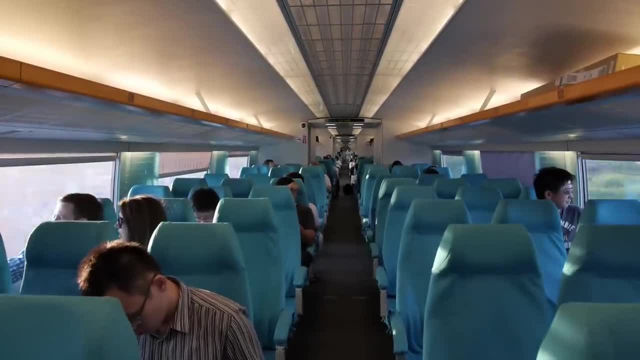 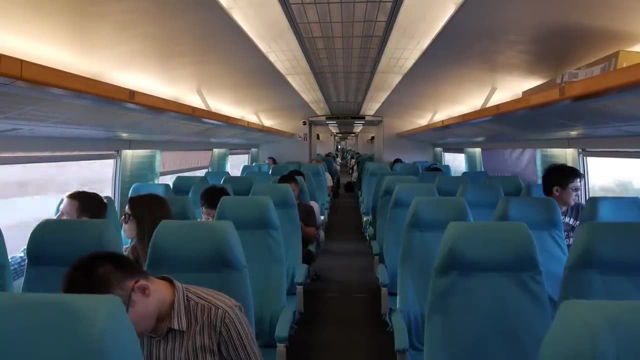 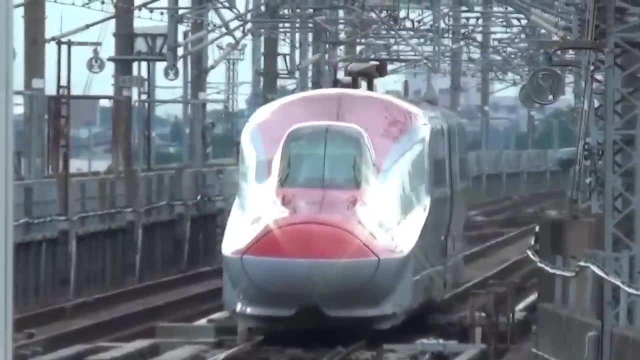 the E5 and H5 can cover the distance of 444 miles, or 715 kilometers, in just under 3 hours. What sets these particular trains apart from their competitors is not only their super speed or price, but also their unique design. The Shinkansen E5 and H5 series have a distinct exterior, which makes 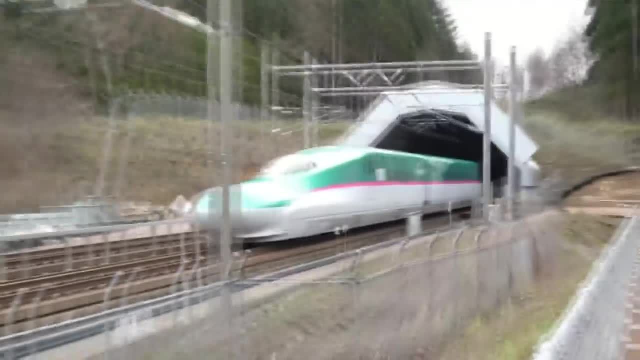 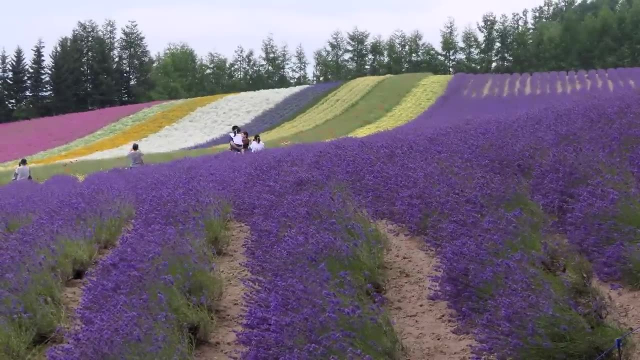 the trains that much more memorable and remarkable. With a green and purple finish, the trains feature images of lilac, lupin and lavender flowers, which have a deeper meaning than just their pleasant design. These beautiful flowers represent the northern and second-largest island of Japan. 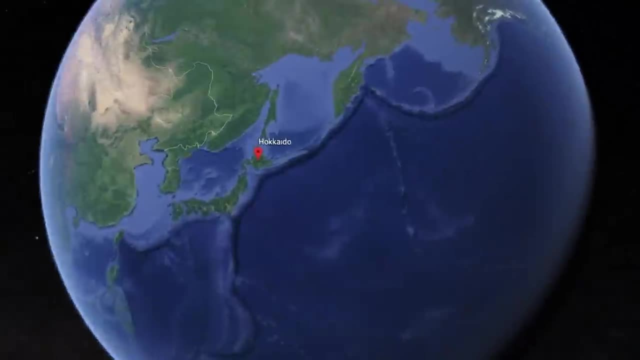 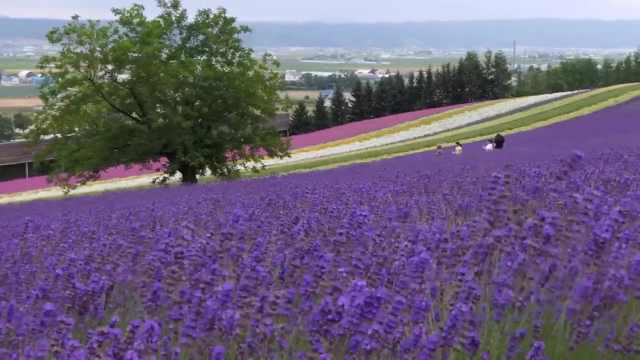 Hokkaido. This island is known for its incredibly breathtaking flower fields and arrangements, amongst which lilacs, lupins and lavenders predominate. But apart from its gorgeous exterior display, Shinkansen E5 and H5 series also have a characteristic 50-foot or 15-meter-long. 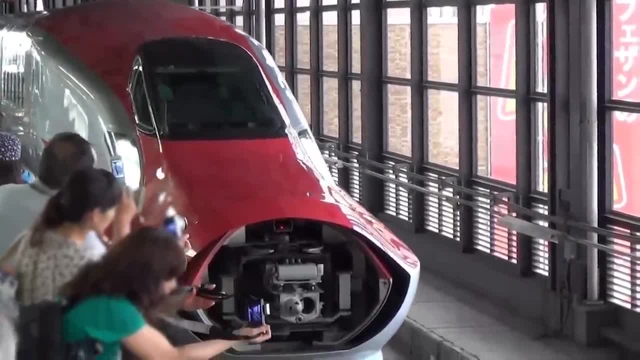 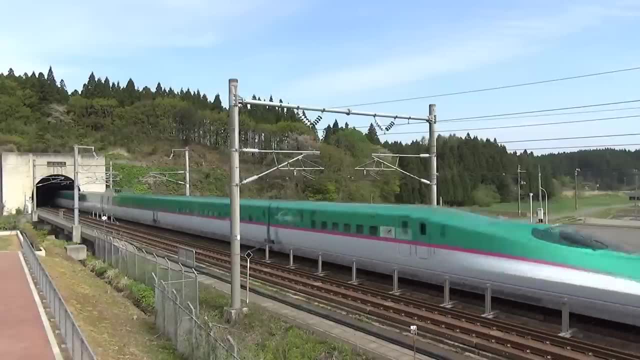 high-speed train which aids in minimizing sound blasts in tunnels, And with active suspension systems installed across the train's length, vibrations of moving compartments are vastly reduced. for maximal comfort. Number 4. Talgo: 350, 227 miles per hour. 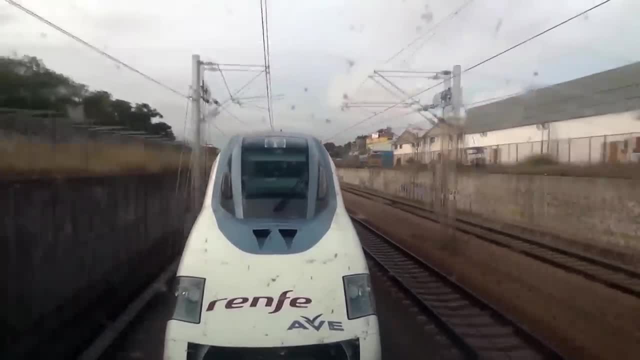 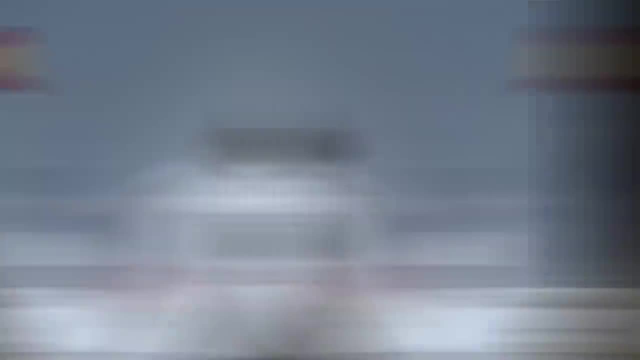 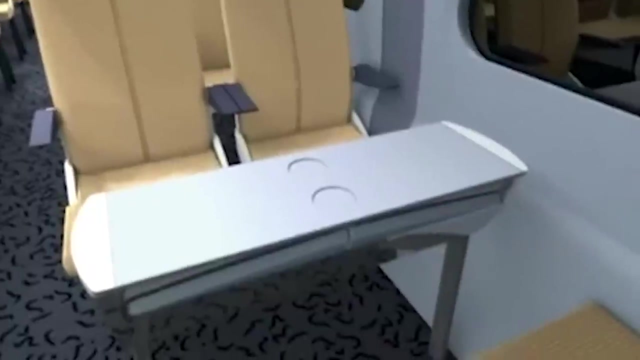 Initially named Renfe AVE Class 102,. the Talgo 350 is one of the fastest trains in the world. The 660-foot or 200-meter-long high-speed train has connecting lines in Madrid and Valladolid and has been an active mode of transportation from 2007.. The Spanish-constructed train has 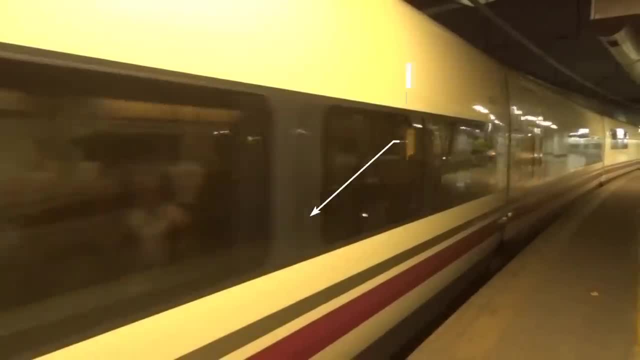 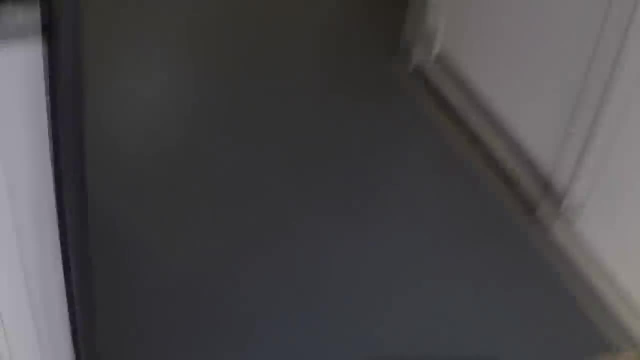 an innovative technology which allows it to reach a speed of 227 miles per hour or 365 kilometers an hour. With Talgo's signature lightweight material, the 350 model offers railway operators high performance and efficiency with each train ride, not to mention its airtight and pressurized body. 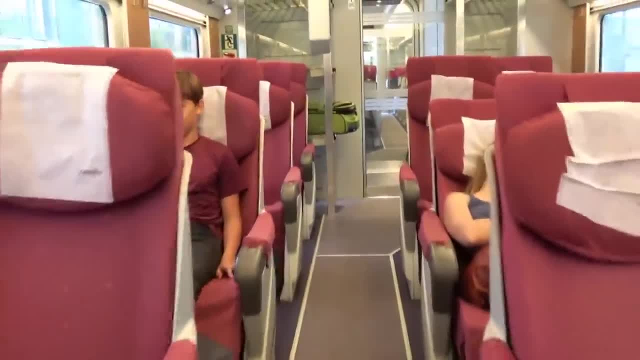 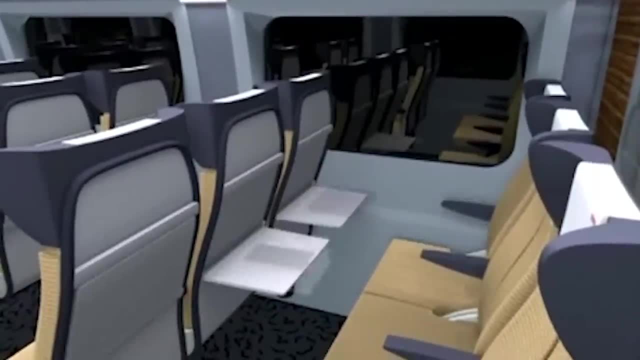 which provides comfortable passes through tunnels and crossings. The seating arrangements are divided into four classes, and the Talgo 350 has a maximum capacity of 1,219 feet, The most powerful of 400 travelers at a time, With equipped video and audio devices at each seat. this high-speed 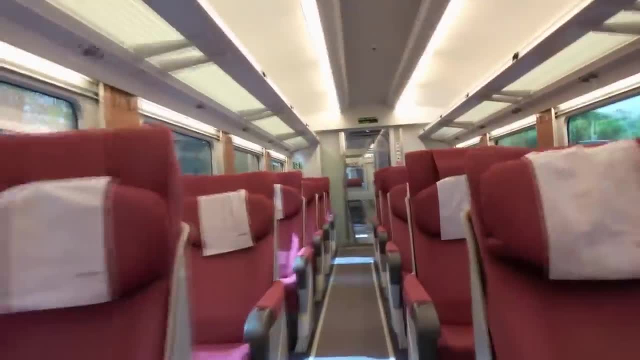 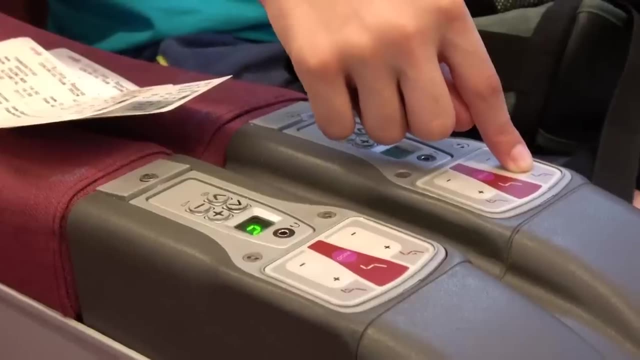 train can be efficient and entertaining at the same time. If you enjoy a good book during your relaxing train ride, then you can use the reading lamps attached to cabin tables. As for electronic devices, power outlets are provided at individual seats, which enhances every passenger's comfort. 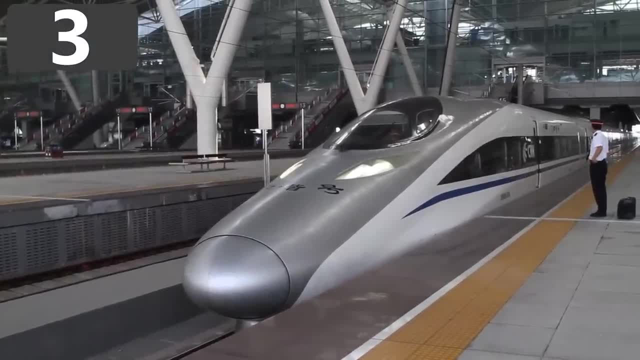 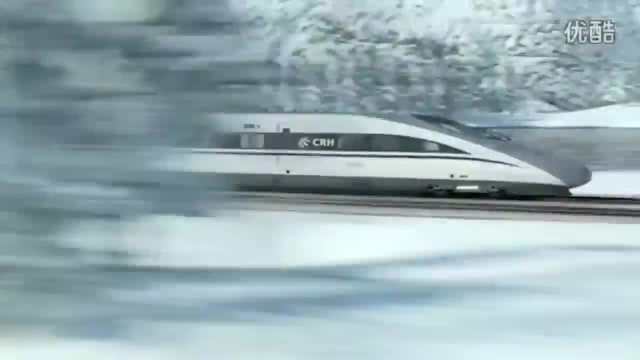 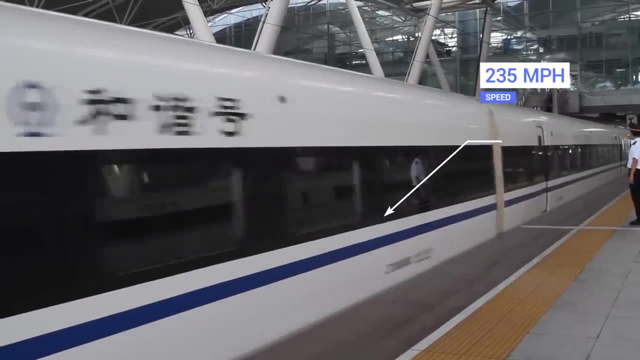 3. Harmony CRH380A, First in service since 2010,. the Harmony CRH380A is China's fastest train up to date, With a maximum lightning speed of 235 mph or 380 kmh. the third-fastest high-speed train in the. 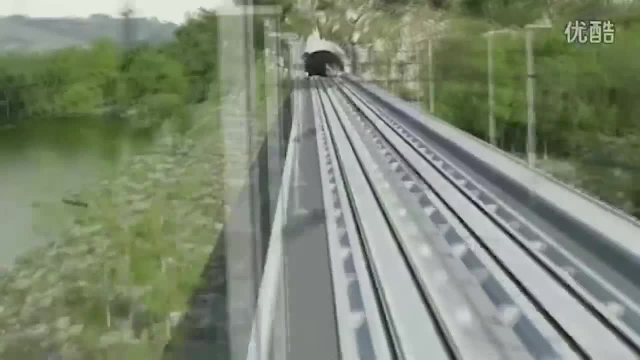 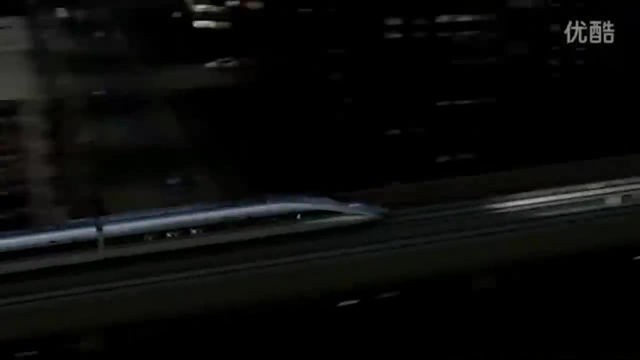 world operates from Beijing to Shanghai and has many stops in multiple cities and towns. The longest high-speed line in China is also notorious for its meticulous design and careful detailing. The design work was carried out in four main categories and it took more than five years. 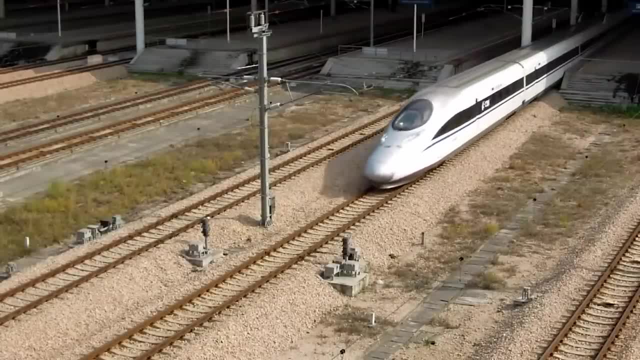 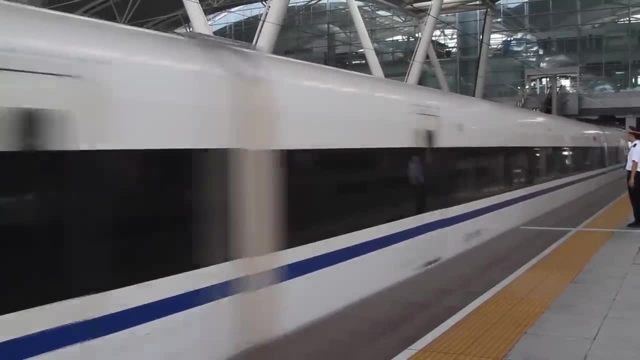 to perfect the optimal design. The high-speed line in China is also notorious for its meticulous scheme and model, But when it comes to stunning fast speed, the technology that was used to reach the maximum speed was discovered through thorough research. These studies were carried out at various 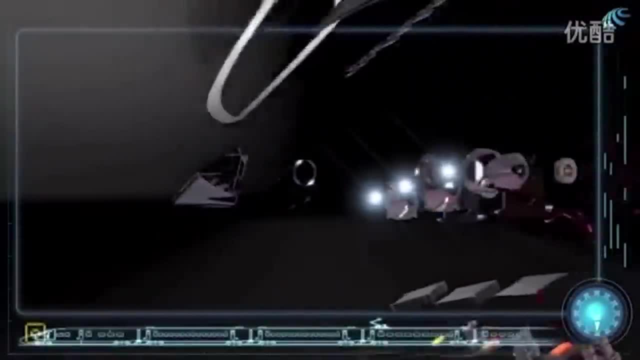 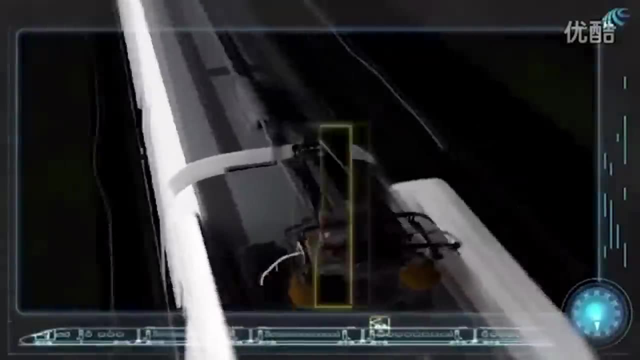 universities in China and were ultimately used to tweak and improve the final CRH product. The Harmony CRH380A serves its name right because this modern train was designed to be completely vibration-free. Train cabins and internal structures were built in such a powerful way. 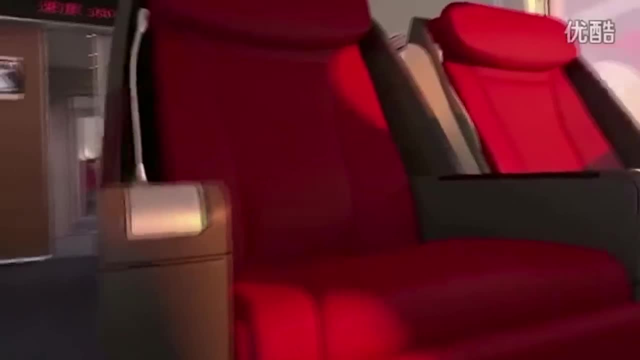 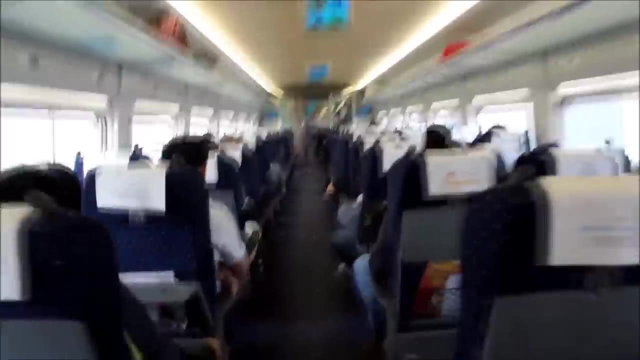 that they can withstand a stunning maximum speed of 340 mph. 3. Harmony CRH380A. The Harmony CRH380A is the world's fastest high-speed train in the world. It has a maximum speed of 350 mph and with advanced noise control technologies incorporated in the overall design. 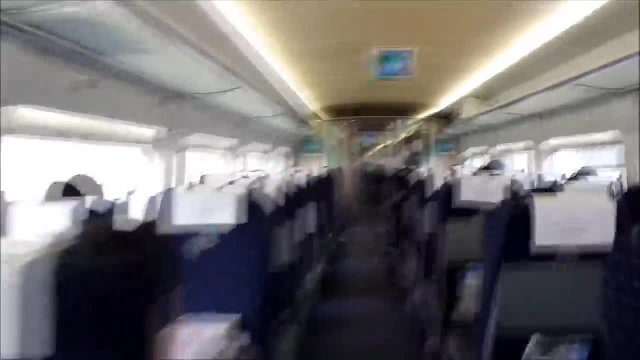 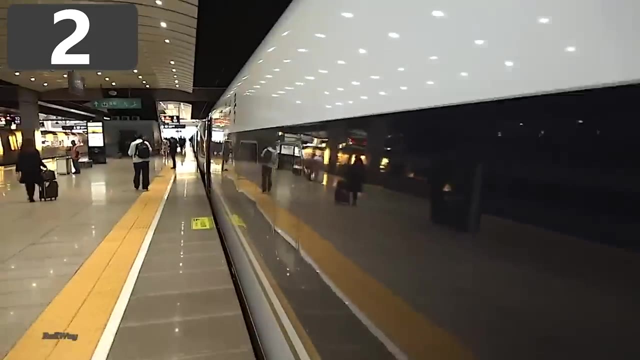 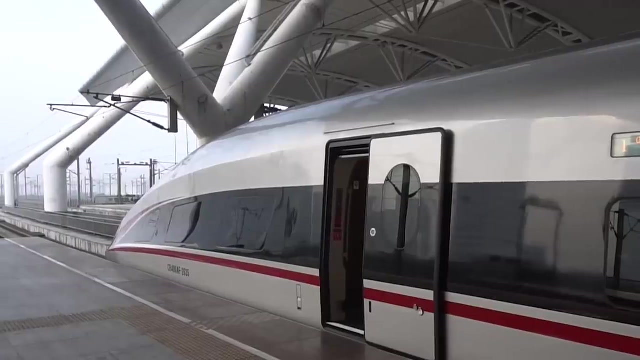 the Harmony CRH380A model has sound-absorbing and eliminating properties like no other. 2. Fuxing Hao: The silver medal for the fastest high-speed train in the world goes to the Fuxing Hao CR400AF, officially introduced into service in June of 2017.. The China railway-operated train travels. from Beijing to Shanghai and is the world's fastest high-speed train. in the world, The extraordinary bullet train can run faster than the Japanese Shinkansen models and has a jaw-dropping speed of 249 mph. The signature bullet-nose aerodynamic design reduces 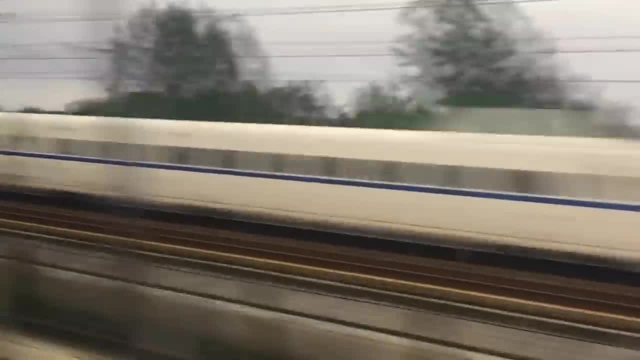 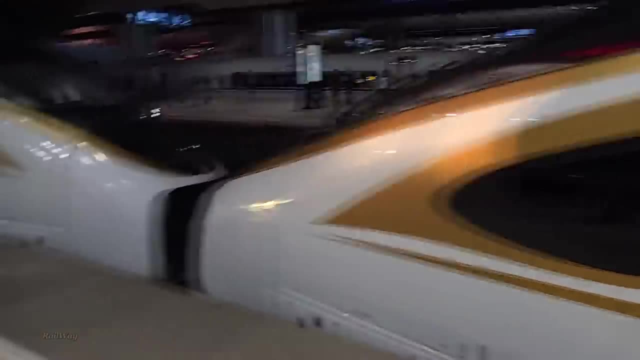 air resistance, which aids with overall high speed and efficiency. The Chinese constructed train has two configurations, one being the standard 8-cart version, while the other is twice in size and is a 16-cart model, With a maximum capacity of 556 and 1200 v. the train is 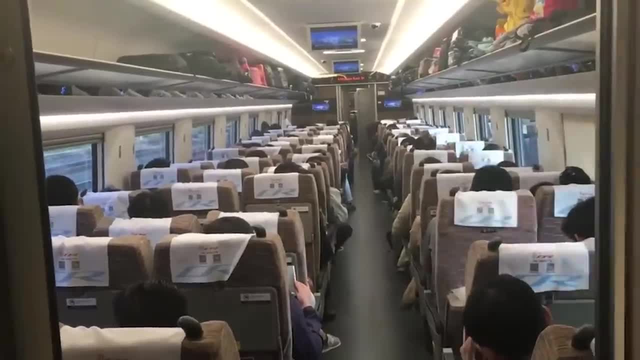 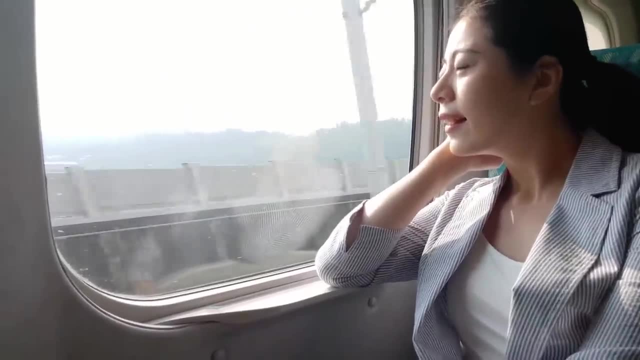 capable of carrying up to 1,200 passengers respectively. The Fuxing Hao aims to offer spacious internal cabin space and comfortable experience to all travelers. The second-fastest high-speed train in the world also has a distinct red and golden exterior design. 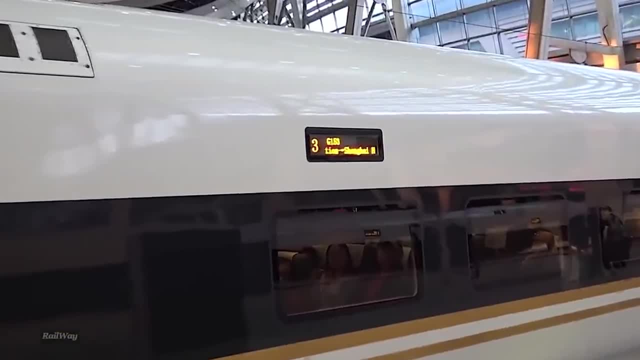 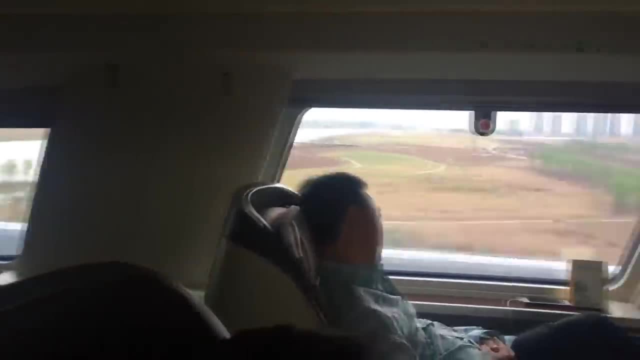 which gives it an edge when compared to its sub-par competitors. If you're traveling in the first-class compartment of the Fuxing Hao, you can turn your seat into a comfortable bed- a perfect option for those sleepless and restless nights. 1. Shanghai Maglev. 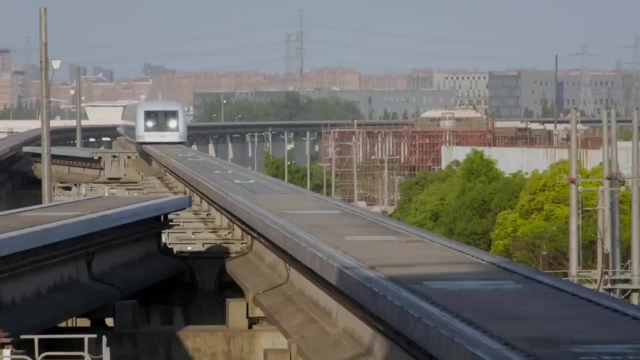 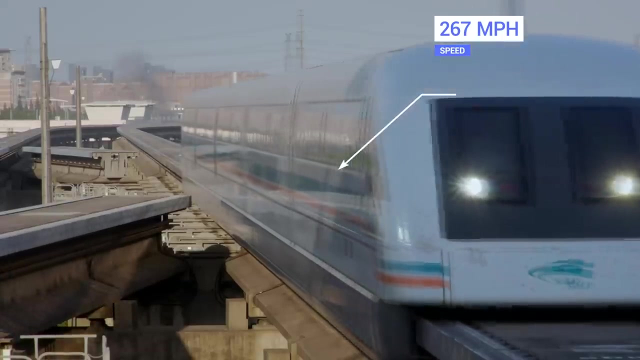 267 mph. Behold, the fastest high-speed train in the world is the Shanghai Maglev, With a shocking speed of 267 mph. the speed of the Shanghai Maglev is unmatched by its inferior train competitors. The first-ever commercially operated high-speed magnetic levitation line has been in service ever.